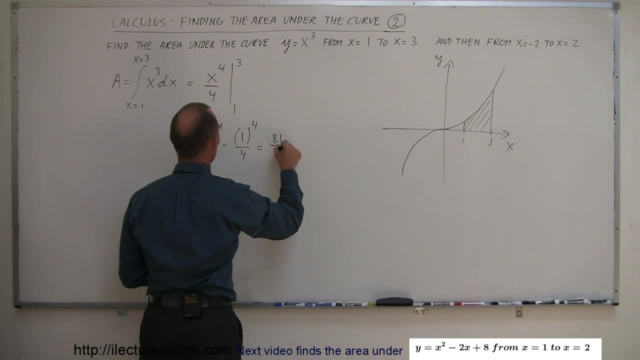 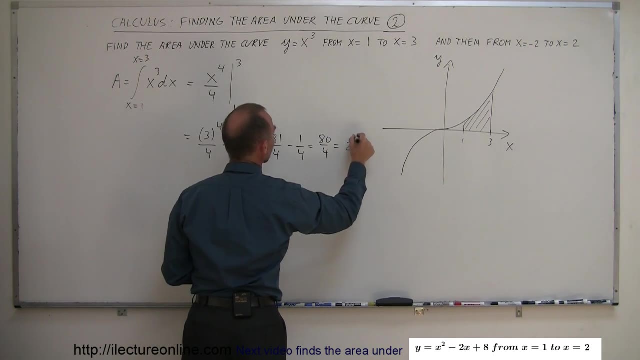 the fourth power, that is 81. So that's 81 over 4 minus 1 over 4, which is 80 over 4, which is equal to 20.. So 20 would be the area underneath the curve for that function. from x equals 1 to x. 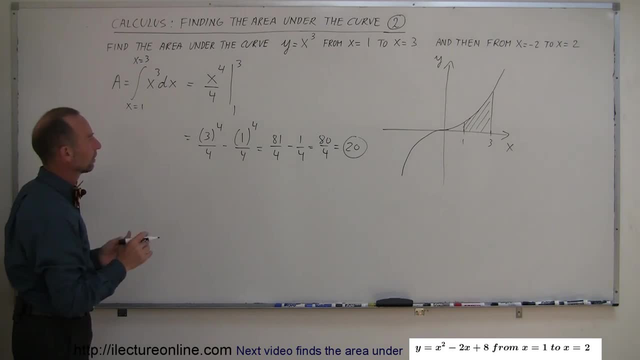 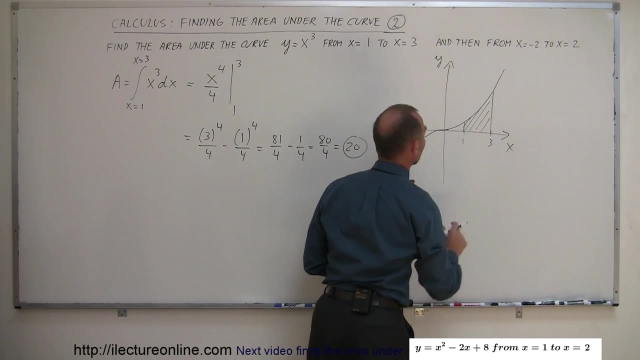 equals 3.. All right, and now for the second part of the problem. we're going to set the limits from x equals to minus 2 to x equals 2.. So let's redraw the graph again Over here. and now the limits are going to be set from x equals minus 2 to x equals 2, and so when? 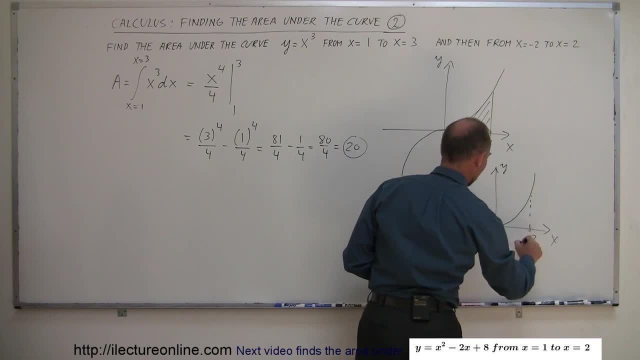 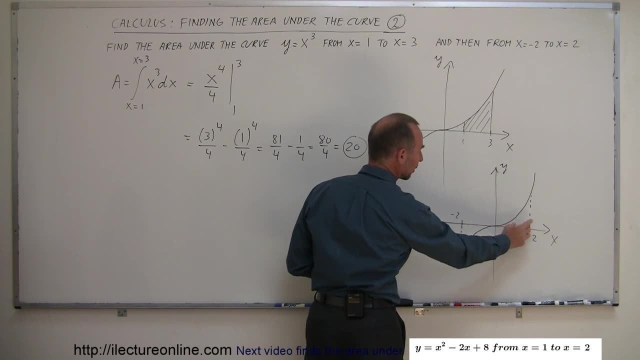 we draw the line like that. draw a line like that. you can see now how there's perfect symmetry. You can assume then that the area here is exactly the same as the area there, but here the area is above the x-axis, here the area is below the x-axis, and whenever the area is below the x-axis. so 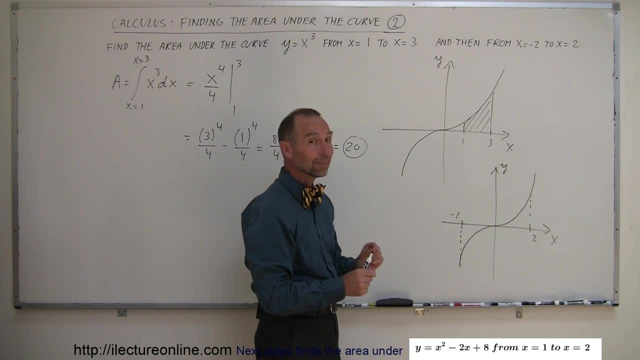 between the curve and the x-axis, but below the x-axis. the area will then be negative. So you're going to get a negative here, you're going to get a positive area there and they'll probably cancel out and get zero. So let's try that. So we're going to find the area when the limits are from x equals minus. 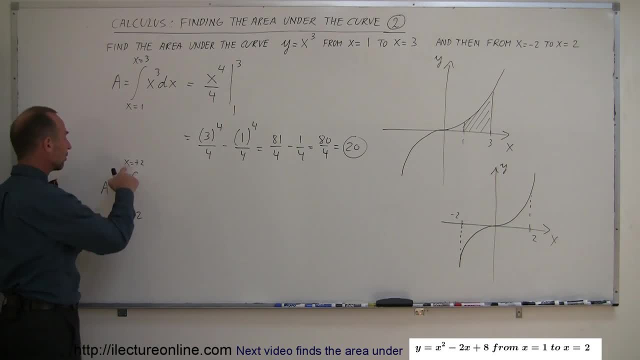 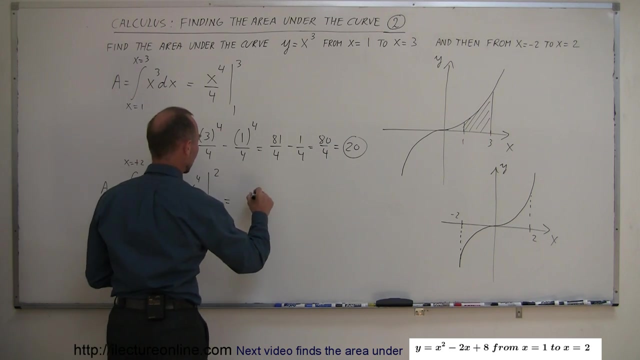 2 to x equals positive 2.. Now I did write x equals, x equals. you don't have to do that, but this is just for clarity of x cube dx. When we integrate that, we get x to the fourth over 4 and we're going to evaluate it from minus 2 to 2.. So first we plug in the upper limit, so we get 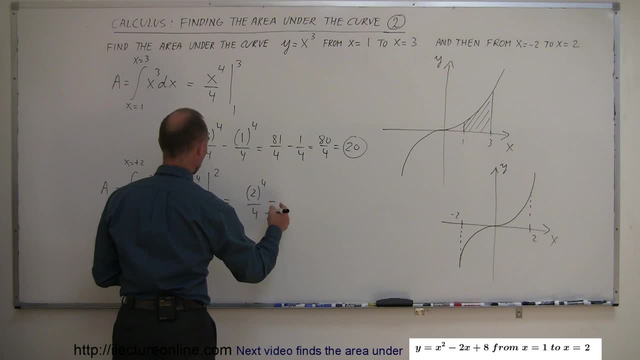 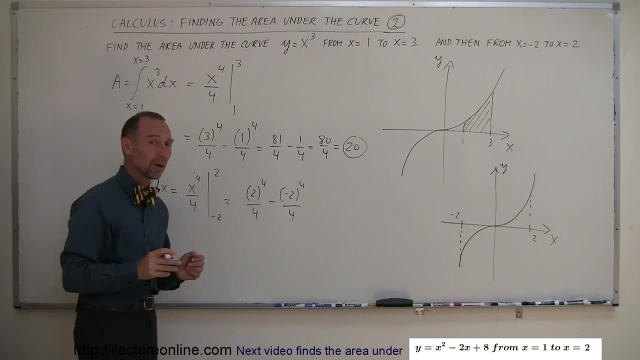 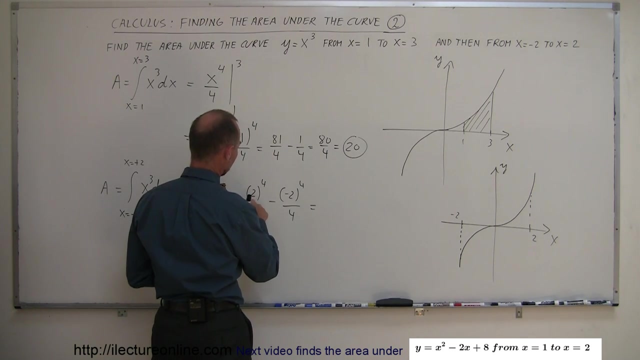 2. the fourth power over four, minus. when plugging the lower limit, which is minus two, to the fourth power over four- and of course, since they are, these are raised to the fourth power. that's an even power. the negative sign doesn't matter, and so this becomes um. two to the fourth power is, uh, eight. 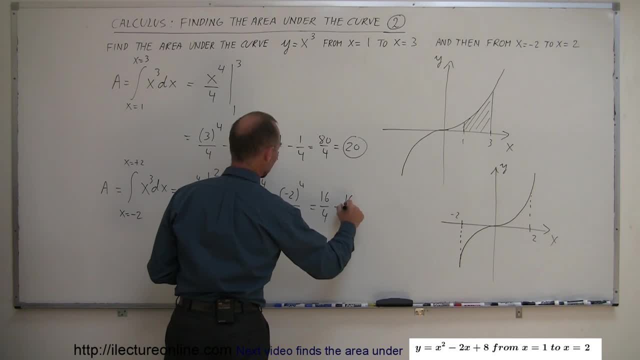 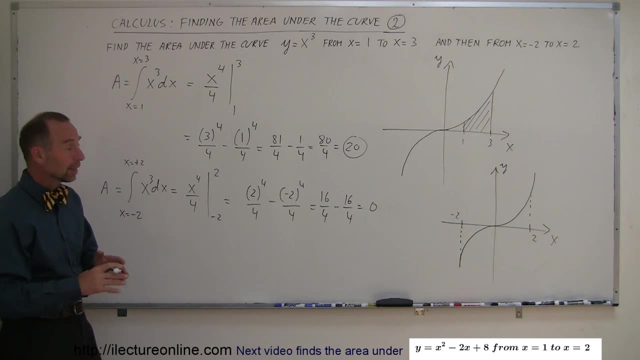 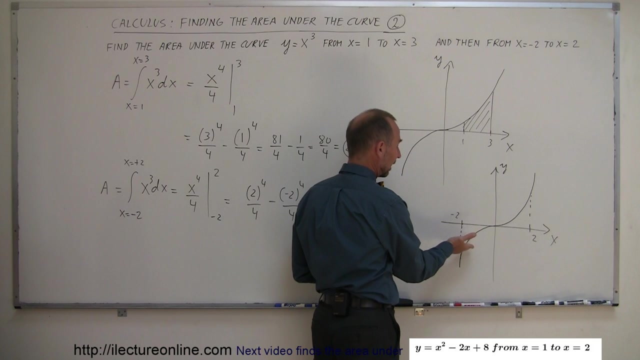 that's sixteen. that's sixteen over four minus sixteen over four, which is zero, just like we predicted. so here we have to be careful. now. that could be the mathematical answer that we're looking for, or we can simply say that the area between the x-axis and the curve could be: